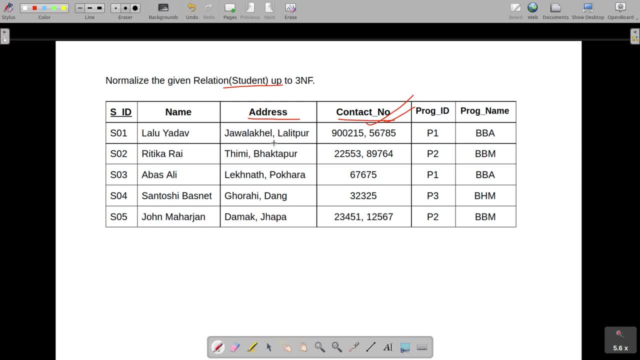 this looks like multi-valued attribute, but if you look closely this is following a certain pattern that is jaulakhel- lalitpur. that means jaulakhel is a part of lalitpur and timi vaktapur leknath. 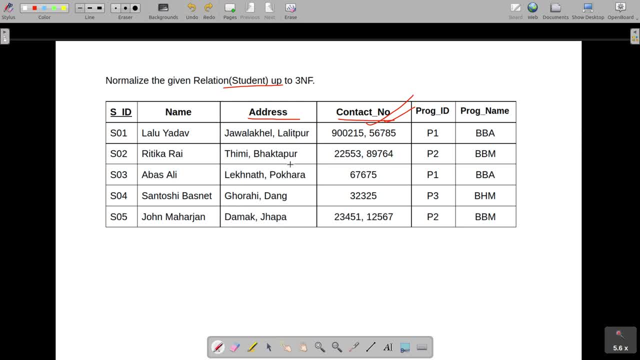 pokhara, gharai dhang and damak dhamak jhapa. so this address is following a certain pattern and there is- it seems like this is like city and district name- timi vaktapur, but this part is not. pokhara is not a district. as far as i know, pokhara is not a district, so we can't see a fixed pattern. 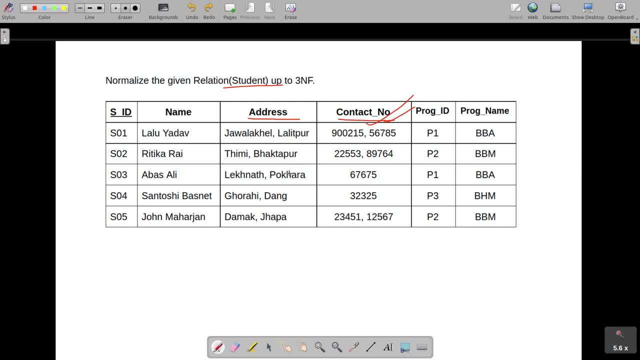 in all the tuples so it is very difficult to break down these attribute in two different attributes. if there was a fixed pattern like rangadi kailali and gharai dhamak dhamak jhapa, if there was a pattern like this, then it would have been very easy to break down this into address city and address district. 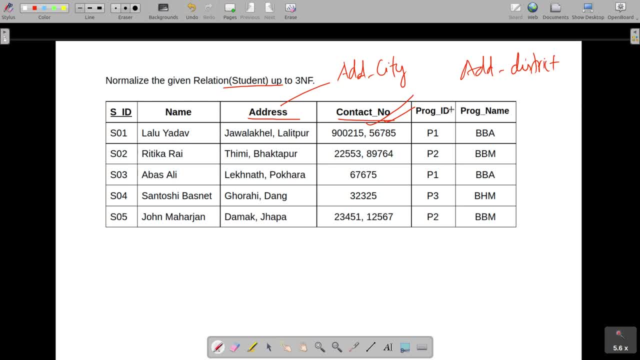 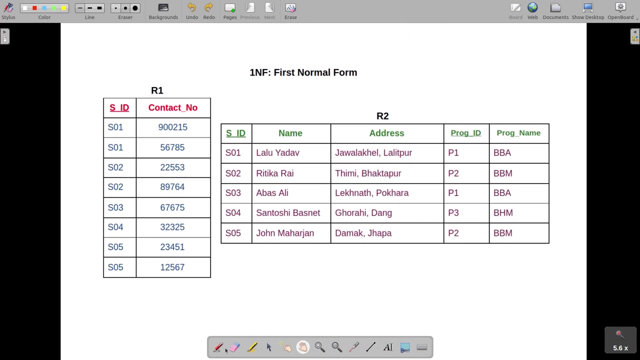 ok, i am saying this would have been, but this is not the case, so it is better to leave it like this. this attribute, this column, does not need to be broken down. so we only take out this in our r1. so in the first normal form, what we do is we have taken out contact number in a different. 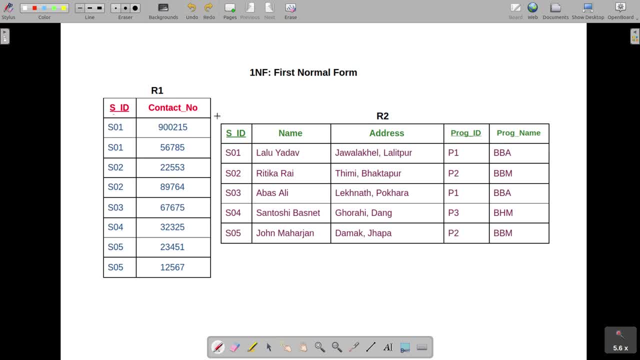 table and here SID remains primary, sorry. SID and contact number- these two mix of SID and contact number remains the primary key here, and in r2 we have SID and program ID. these two are the prime keys. okay, program ID has not been underlined, but since this is a prime key and this is an intermediate table, this 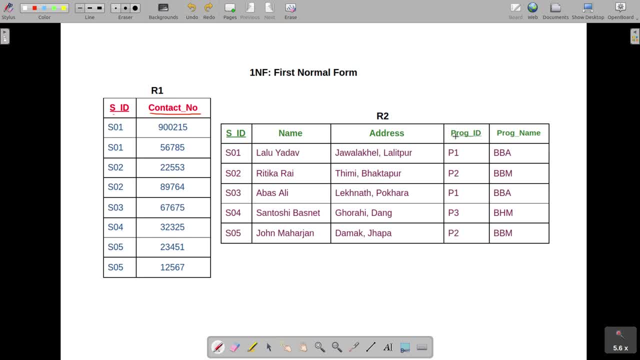 is not the final table we are. we are adding one underline here so that both of them behave as primary key. so this table is fine. now in r2 we have to check if this is in second normal form. okay, we have to now. our target is second normal form after. 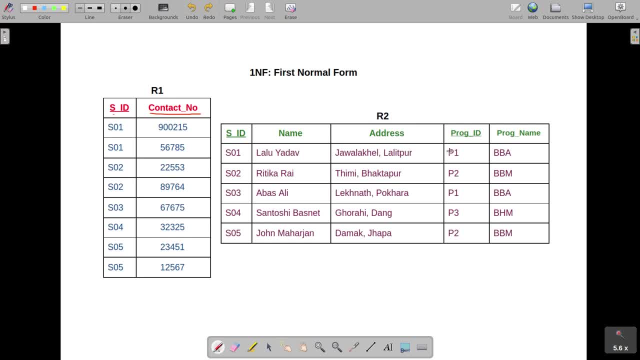 converting the tables in first, normal form. so this is about partial dependency. you see, you have to check if there is a partial dependency, since these two are prime keys- I have underlined these two- and they become the composite primary key, which means all these attributes have to depend on this primary key, both. 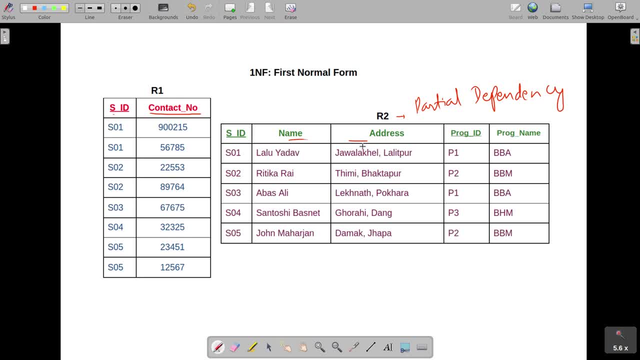 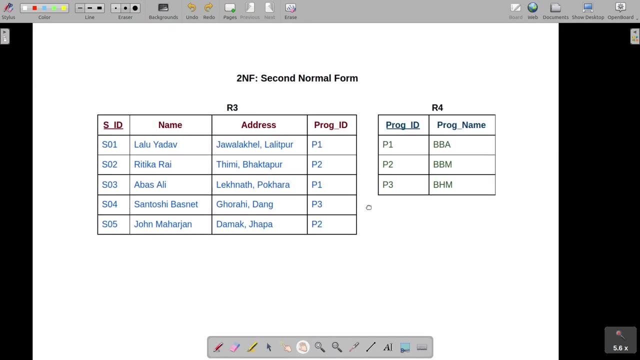 both of them. so these two attributes only depend on s ID and this particular depends on only program id. so let's break down this table. now we have second normal form in which we broke down r2 into r3 and r4. so in r4 we took out program id and program name, program id and program name and 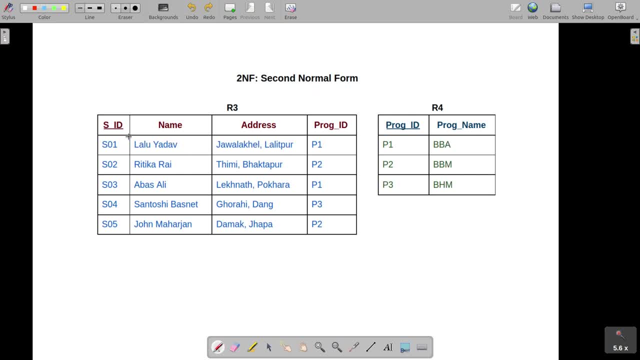 in r3 we have sid and name and address, which depends on sid, which depend on sid and also program id, because we want to have the information which student is enrolled to which program. this information needs to be stored. so we have not removed this column from here. 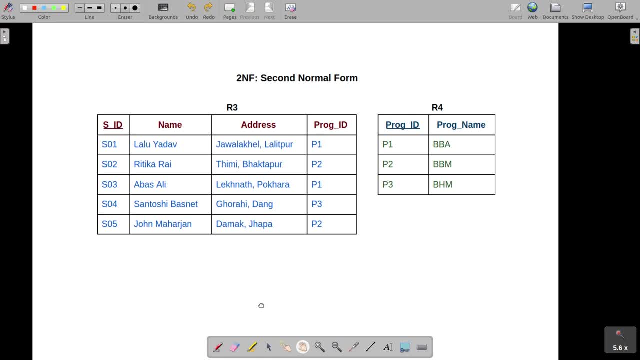 now we have to convert this into third normal form. so now we have the previous r1 table where we have to check for transitivity. now you have to check if there is transitivity here, if there is any transitive dependency or not in r1, r2 and- sorry- r1, r3 and r4.